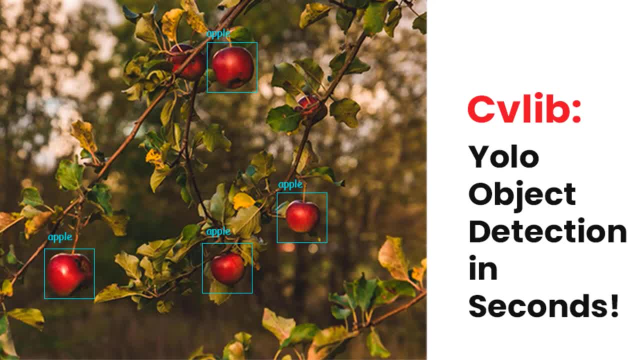 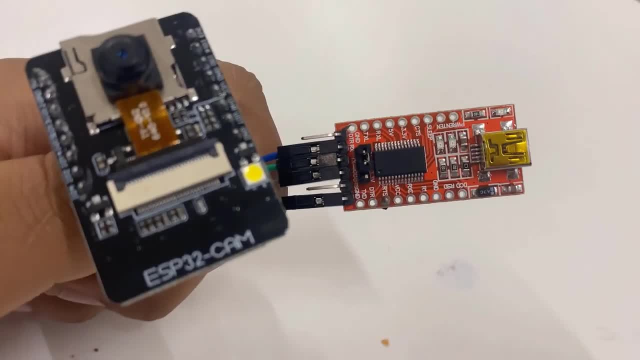 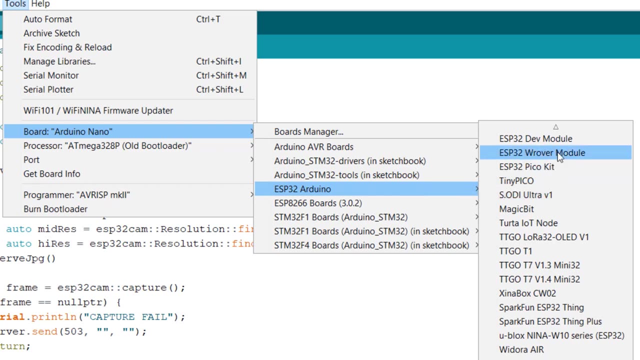 The name of the pre-trained module is YOLOv3.. In this tutorial we will go through its features, pinch descriptions and the method to program ESP32CAM module using FTDI module. We will also set up the Arduino IDE for the ESP32CAM module. 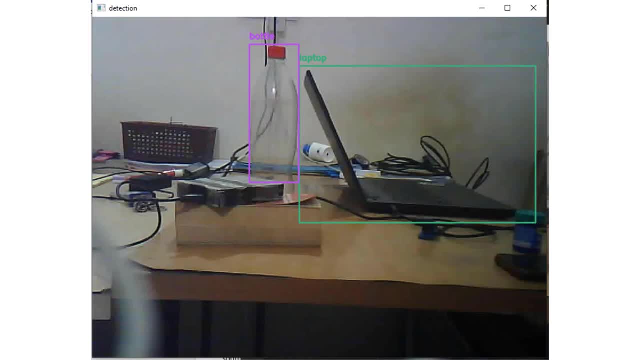 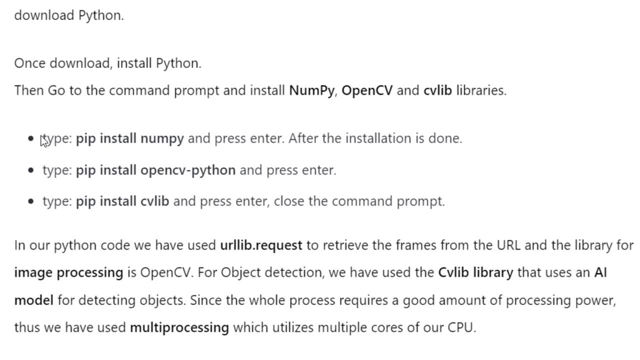 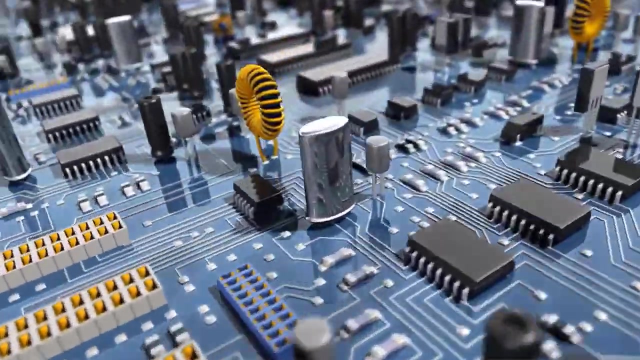 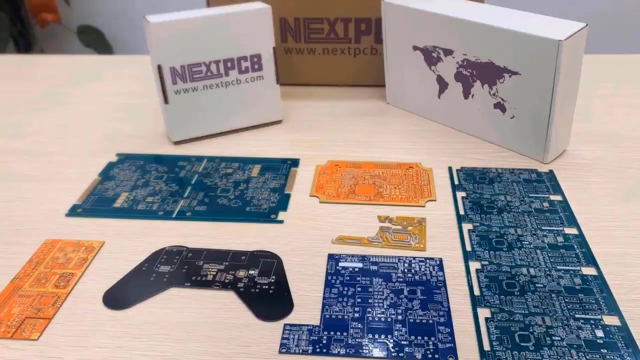 We will also upload the firmware and then work on the object detection. For object detection and identification part, the script for object detection is written in the Python programming language. Thus we will also have to install Python and its required libraries. This video is sponsored by my favorite PCB manufacturer company called Next PCB. 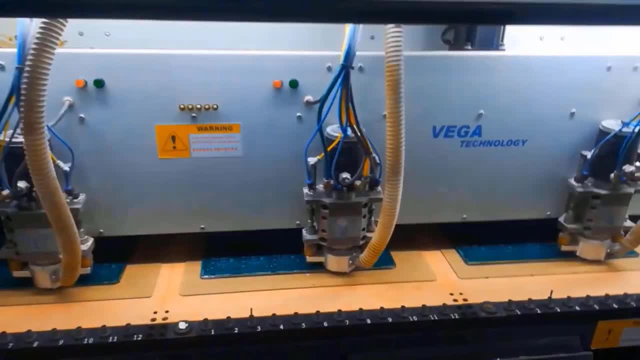 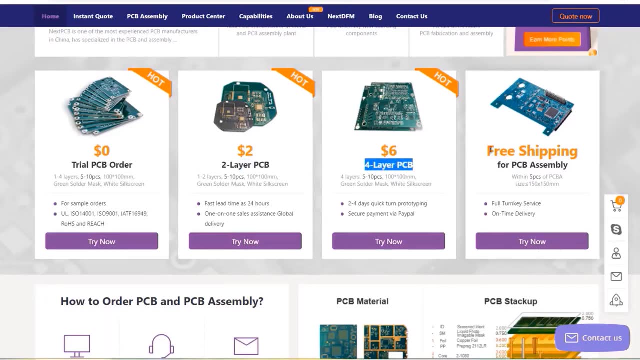 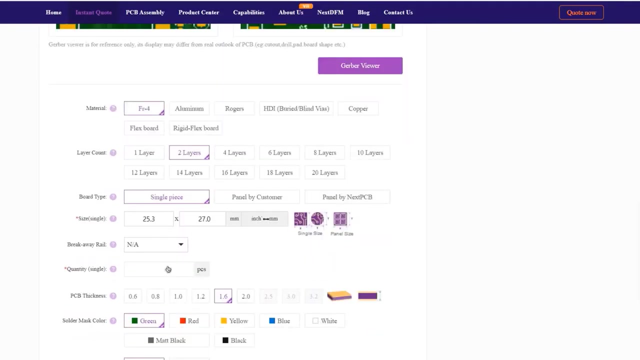 They offer PCB board and PCB assembly services at the lowest affordable price. You can get 12 PCB, 2-layer PCB and 4-layer PCB, with free PCB assembly shipping services up to a fast lead time of 24 hours. All you need is to visit nextpcbcom and upload the Gerber files. select PCB quantity, color, material type and other details. 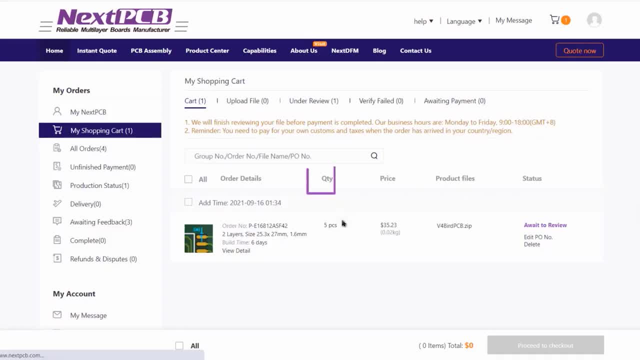 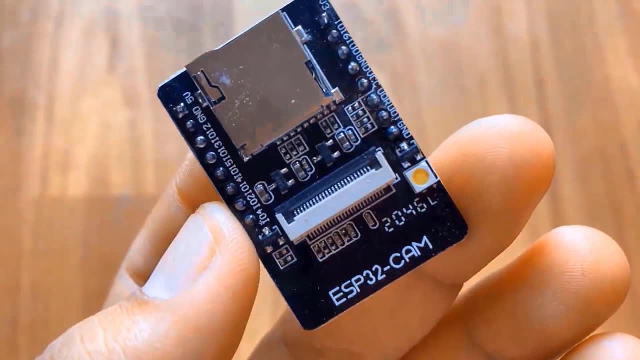 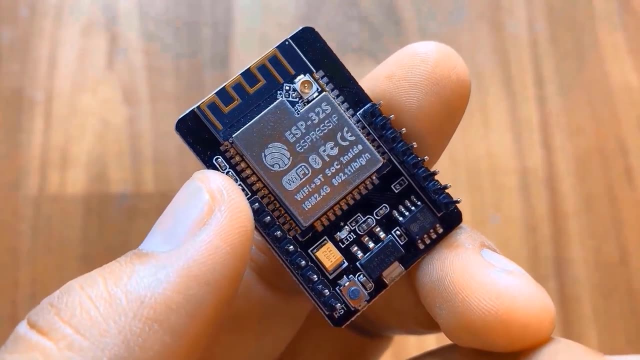 Then press an order. You will get the high-quality PCB within 48 hours. Welcome back again. This is an ESP32-based camera module developed by AI Thinker. The controller is based on a 32-bit CPU And has a combined Wi-Fi plus Bluetooth or BLE chip. 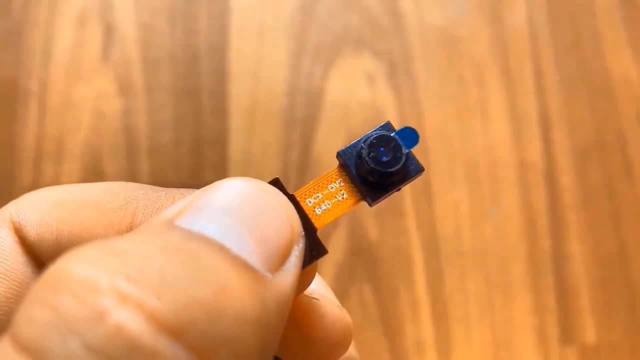 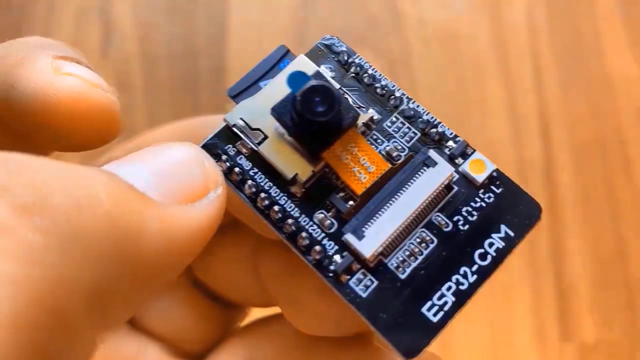 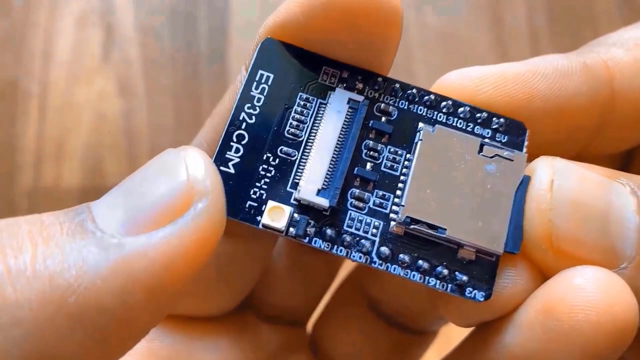 This is the OV2640 camera module, which has the highest camera resolutions, up to 1600x1200.. The camera connects to the ESP32CAM board using a 24-pins gold-plated connector. The board supports an SD card of up to 4GB. 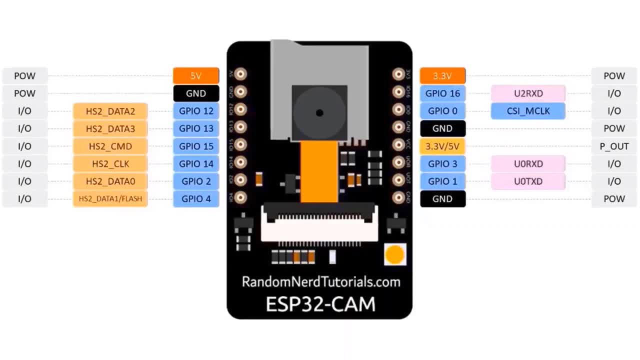 The SD card stores captures images. Its GPIO pins have support like UART, SPI, I2C PIN. The board supports an SD card of up to 4GB. The SD card stores captures images. Itootsy PWM, ADC and DAC. 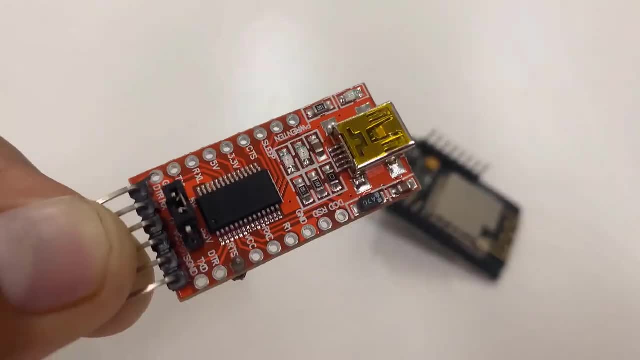 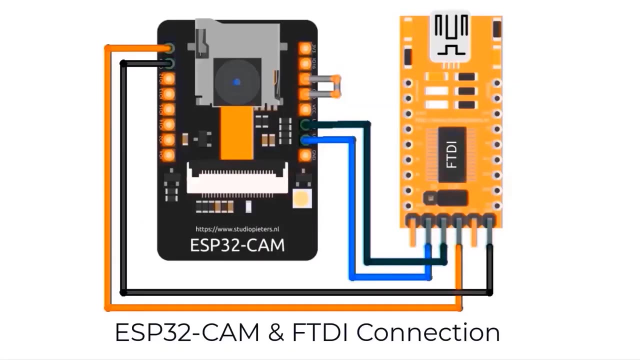 The port doesn't have an on-board programmer, so in order to programme this board, you can use any type of USB-2 TTL module. Please follow this connection diagram for programming and use The programming method and different modes of operations have been explained in earlier videos. 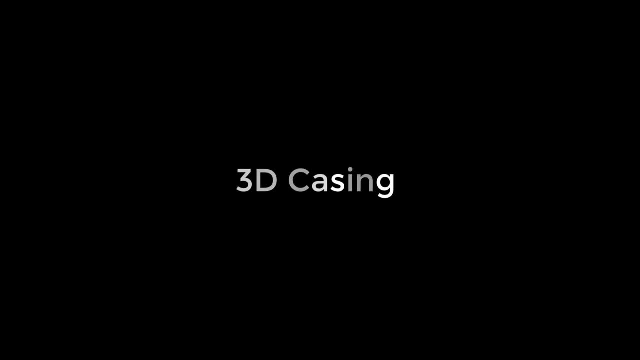 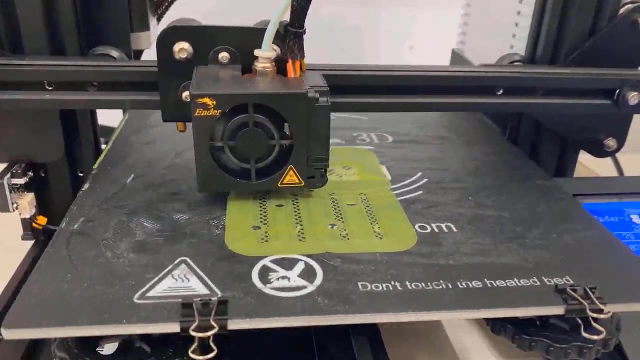 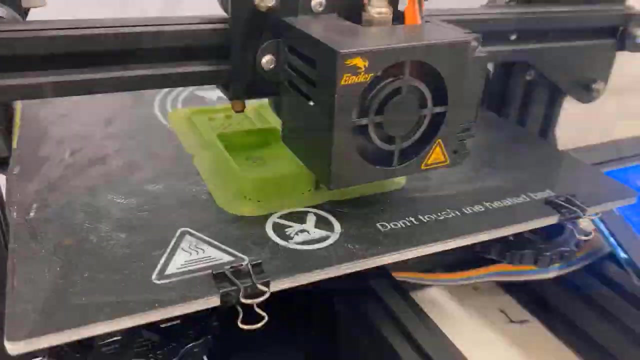 To make this board portable and standalone, I designed a 3-D casing. This is my 3-D3 minded desk. I used solid work to design the 3D casing and then converted the STL files into a Z code. I used my Clarity 3D printer to print all the parts. 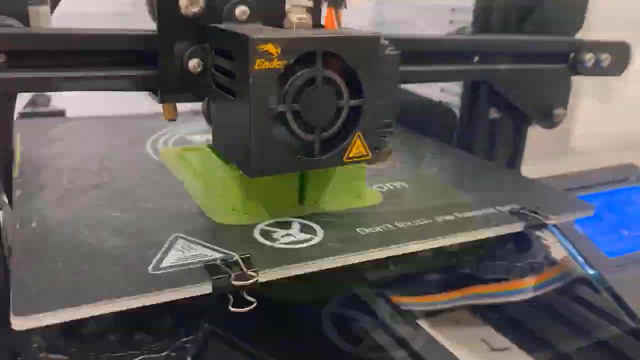 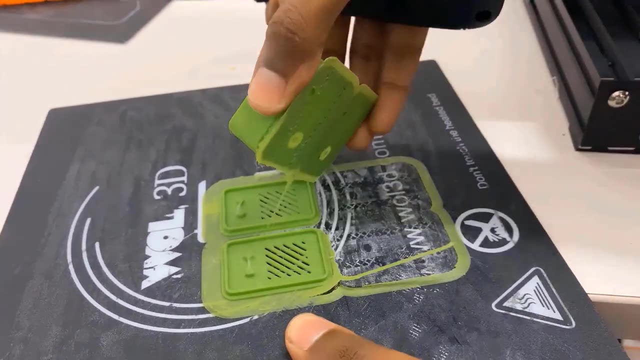 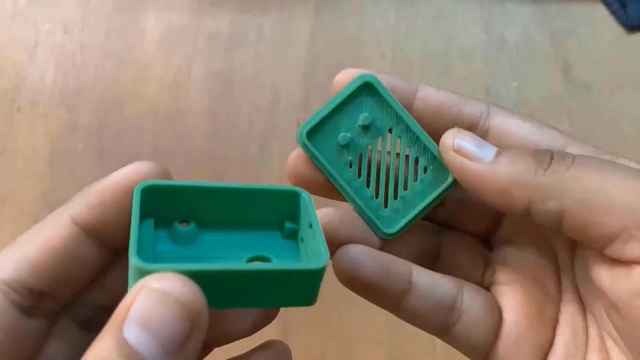 It took nearly 2 hours to print the case. After printing was done, I removed the casing from the surface and eliminated the useless extra support part. This is a pair of casings but both have a different height. The enclosures can be closed using a button part that fits perfectly on the casing. 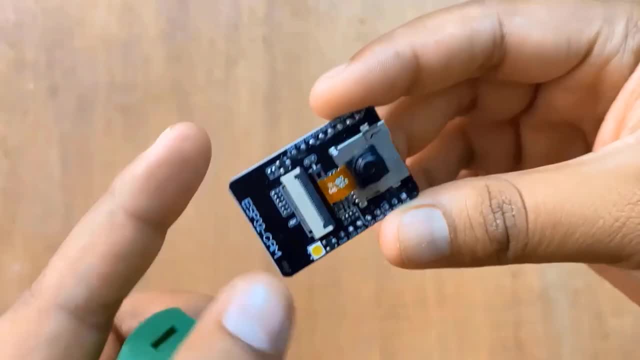 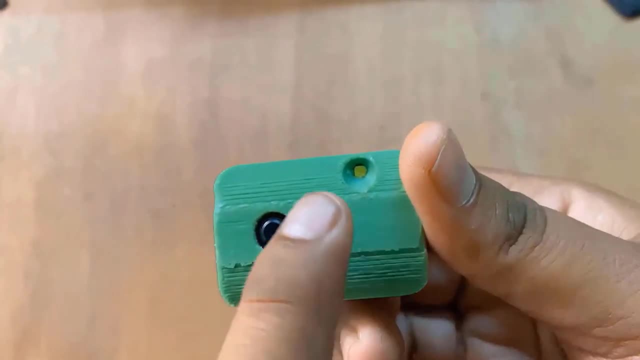 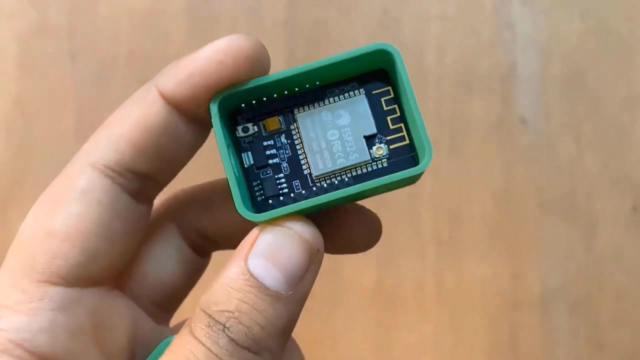 Alright, it's time to fit the ESV32 cam module. There is a hole in the casing, one for the camera and other for the LED flash. You can simply insert the cam module and tighten it. A small battery, probably lithium or lithium polymer, can be installed here inside the box. 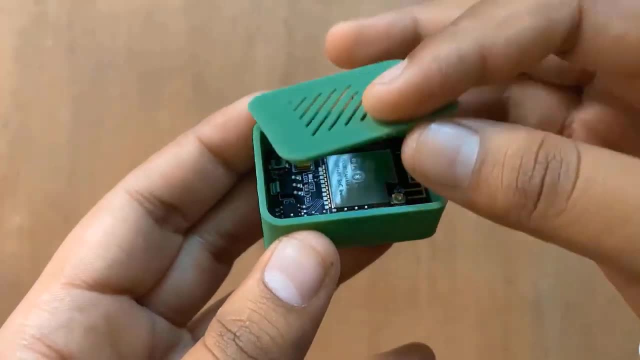 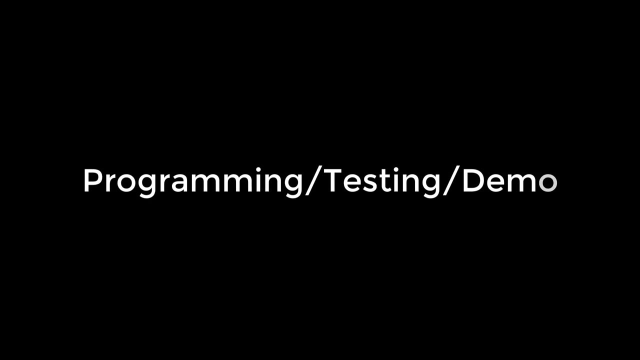 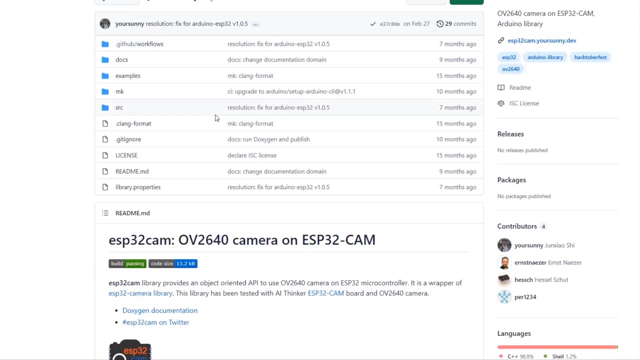 to power on the entire circuit. I am not using any battery right now, as I will like to power it through the USB port. Let's move to the project part now. This project uses a code from ESV32 cam library created by your Sunny. 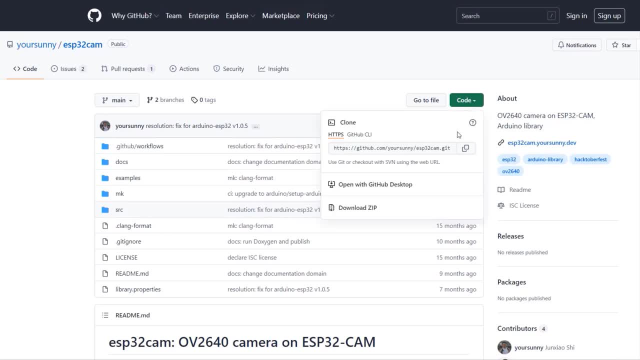 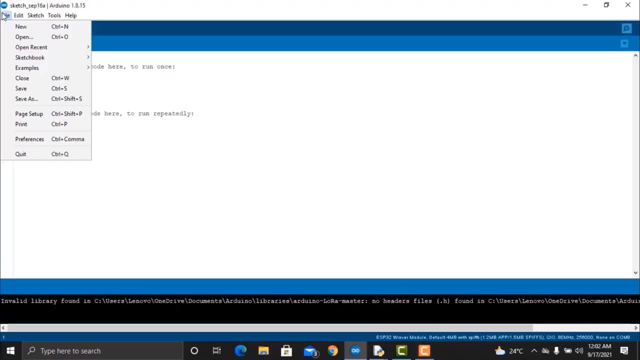 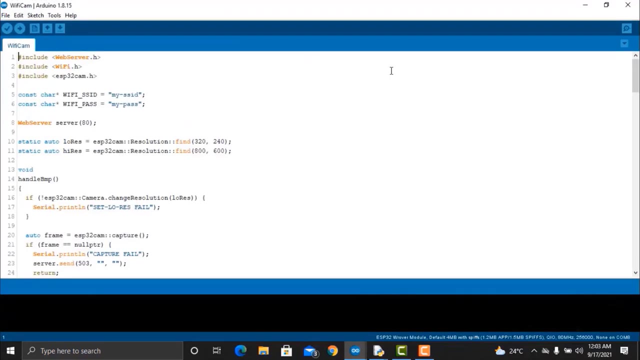 This library supports ESV32 cam and OV2640 camera. You can download the zip file and add it to the Arduino IDE using library manager. Now open your Arduino IDE and, from example, open a file called Wi-Fi cam. In this example, you just need to change the Wi-Fi SSID and password. 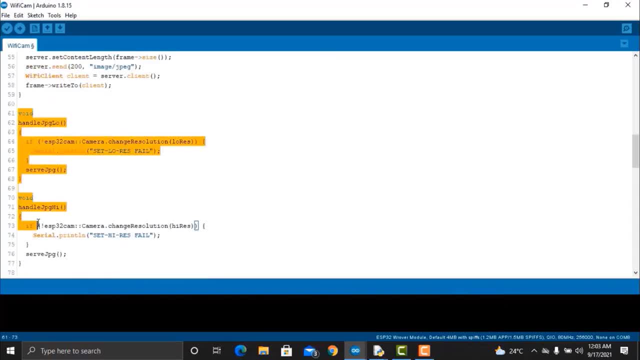 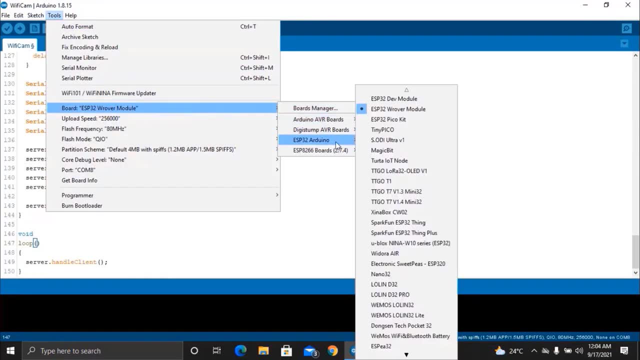 Now open your Arduino IDE and, from example, open a file called Wi-Fi cam. In this example, you just need to change the Wi-Fi SSID and password. The code is the same as for the previous projects. To upload this code, select the ESV32 robot module from the board list. 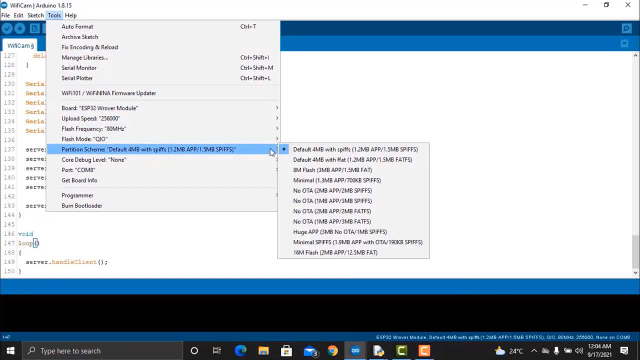 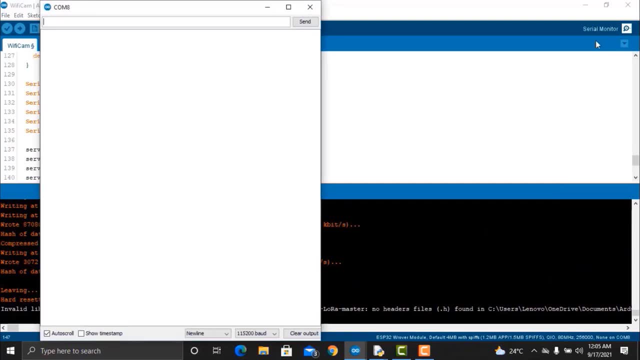 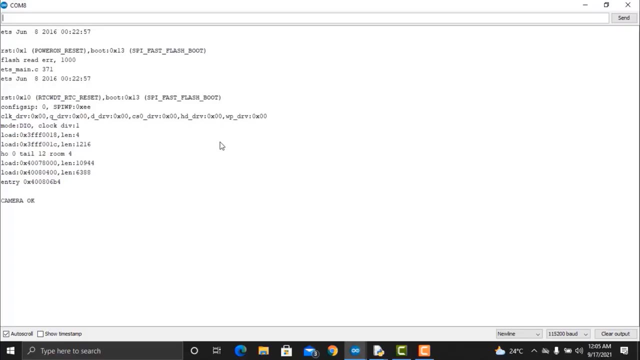 Also select the com port, then click on the upload button to upload the code. Open the serial monitor. once code uploading is done, then remove the shortening jumper and press the reset button. If everything is fine, then you will see the camera open. 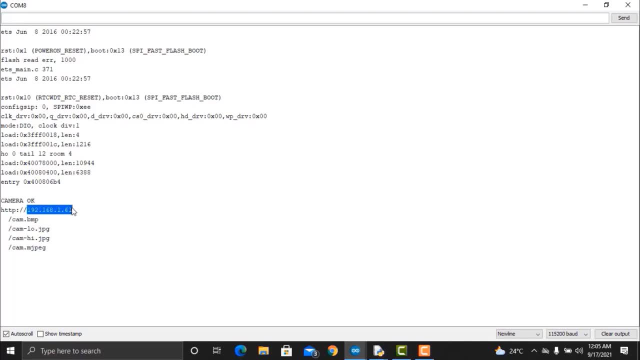 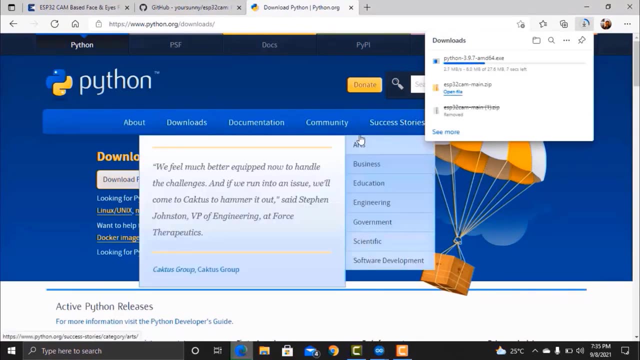 Let's go to the next step. The OK message on the serial monitor and the local IP address of the camera will also be printed. Now go to your web browser and download the Python latest version. Python is required because the machine learning and image processing part is done by Python. 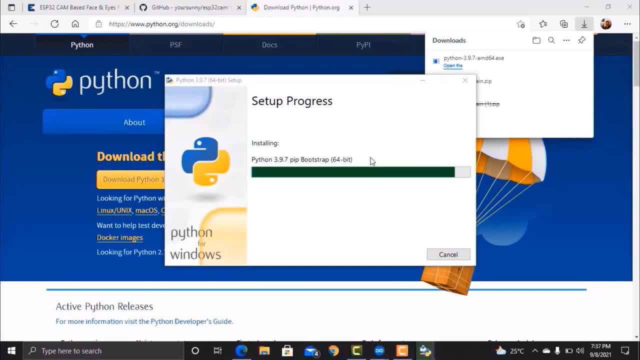 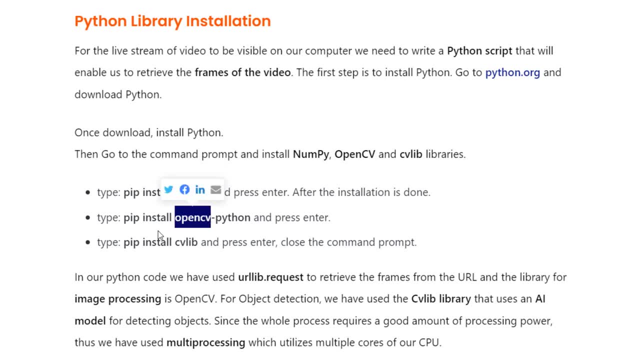 libraries After the Python gets downloaded, complete the installation process. Now we need to install two Python libraries on our operating system, That is, NumPy, OpenCV and Cvlib libraries. Follow the website's article. You will see the article of how to electronics to install the required Python libraries. 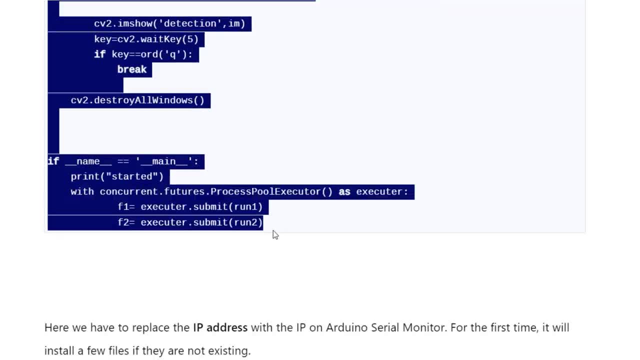 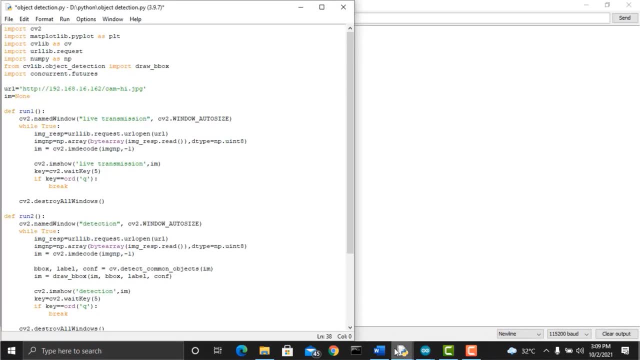 Copy the following code and paste it on any Python editor. Copy the IP address from the serial monitor of Arduino IDE and replace this IP address in the Python editor code. In our Python code we have used urlibrequest to retrieve the frames from the URL and the. 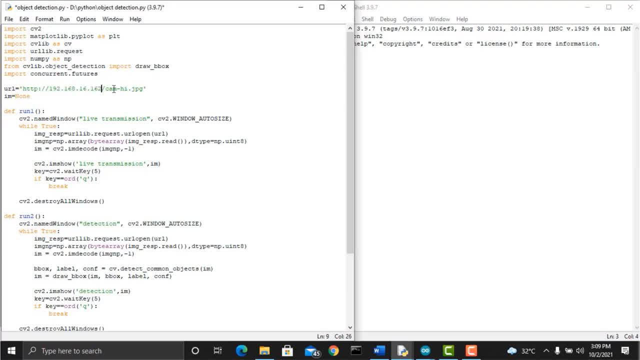 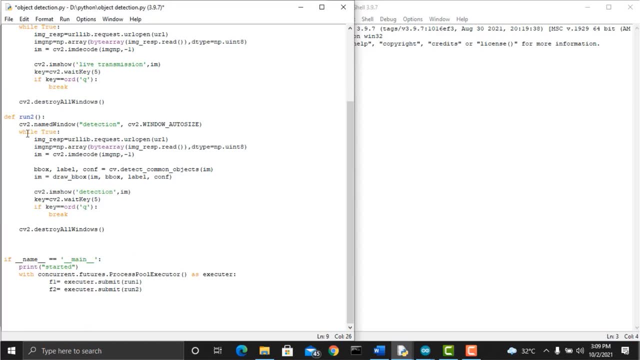 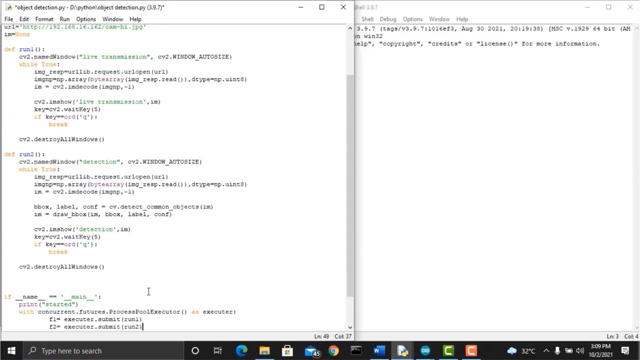 library for image processing is OpenCV. For object detection, we have used the Cvlib library that uses an AI model for detecting objects, Since the whole process requires a good amount of processing power. thus we have used multiprocessing, which utilize multiple cores of our CPU. 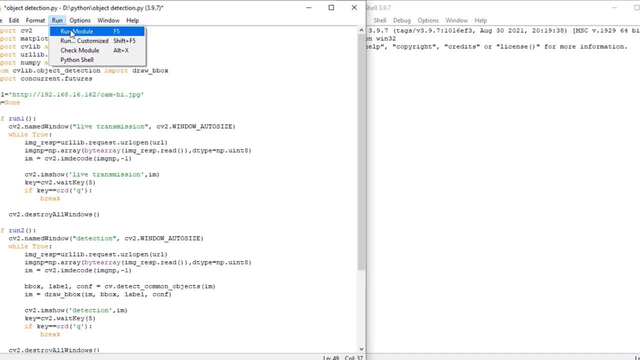 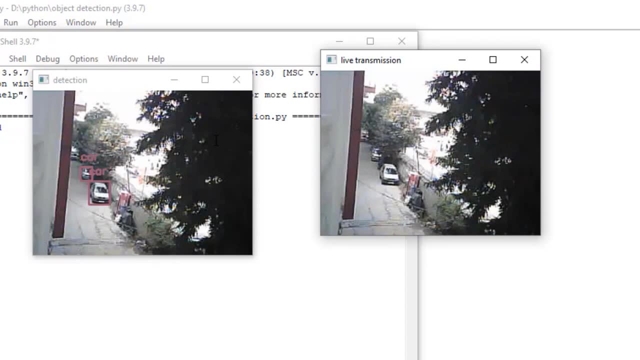 Go to run and then click on the run model option. Once you hit run for the first time, it will install a few files if they are not existing. Once we have done that, we can see two windows named lift transmissions and detected is visible. 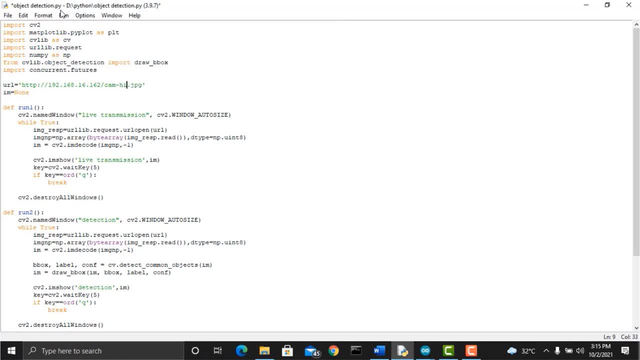 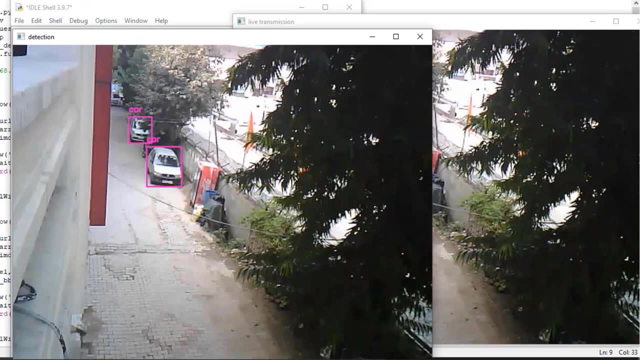 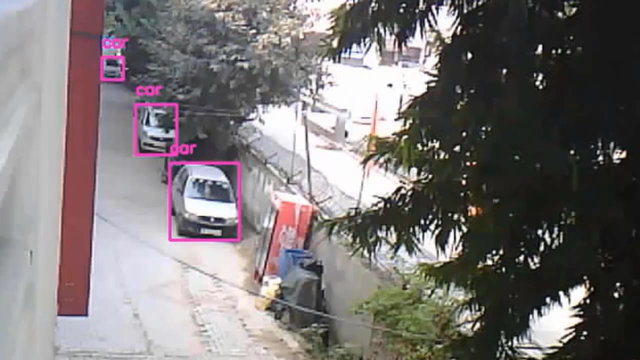 Now in the detected window, one can view different detected objects, as around them, different color boxes are visible. For example, I can see two cars here, which is easily detected by our system. This is how you can use the ESP32CAM along with OpenCV for object detection and identification. 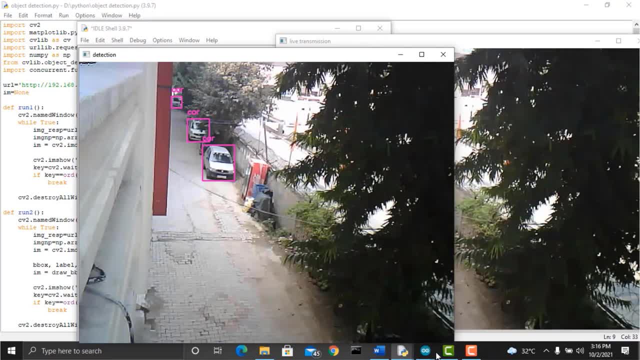 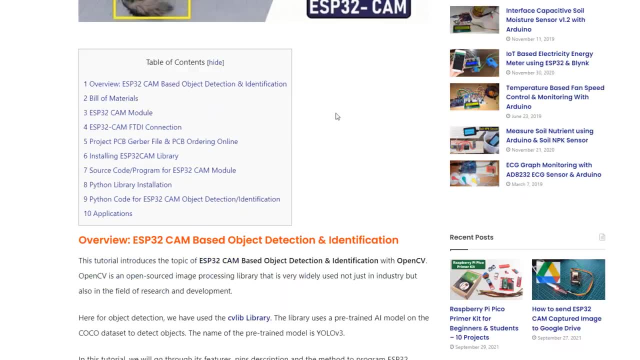 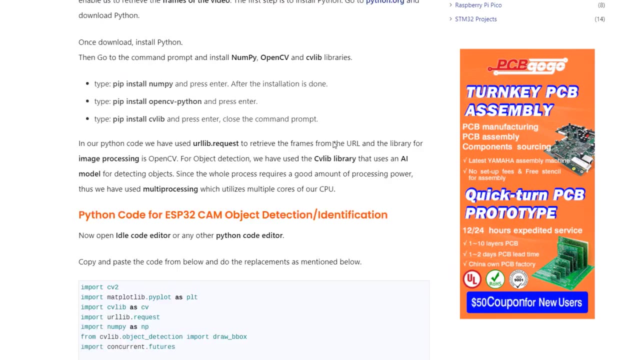 This project can be implemented at an advanced level along with the applications of machine-learning and AI. All the documentation, libraries, details, code and written explanations of this project is perfectly documented on HowToElectronics. I hope you like this video, so please drop a like and subscribe to the channel.